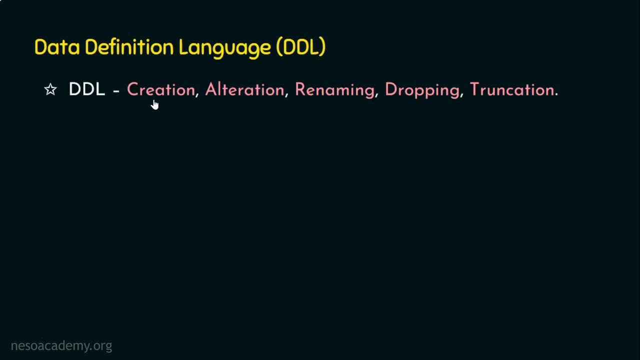 table structure. then creation: we need to create a table. Let's assume we have created a table and we want to modify the schema of the table. After creation of the table, we might be adding a new column or dropping a column, or even altering the type of the existing column. So that is. 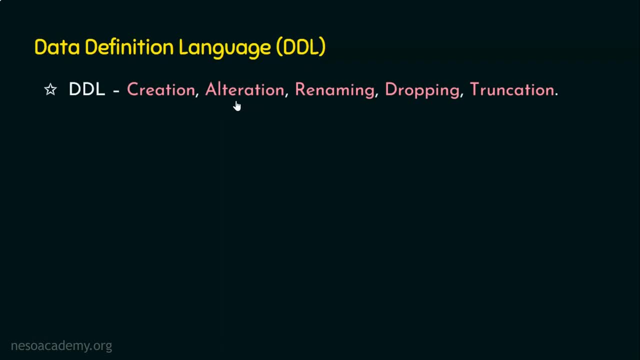 also possible using DDL. So creation of the table, also alteration of the table, Then if you want to rename the table name again, this is renaming the schema only. So this is also DDL, And dropping the table means just removing the complete information about the table, Even the table itself. 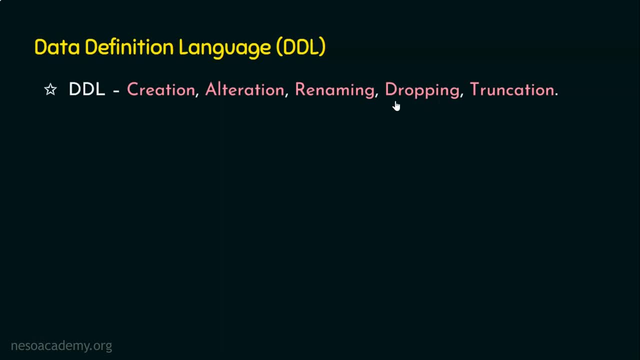 will be dropped from the memory. So the complete removal of the table structure is dropping. Dropping a table means deleting all the data present in the table into including the structure, the schema of the table, And truncation means it's going to delete all the data present in. 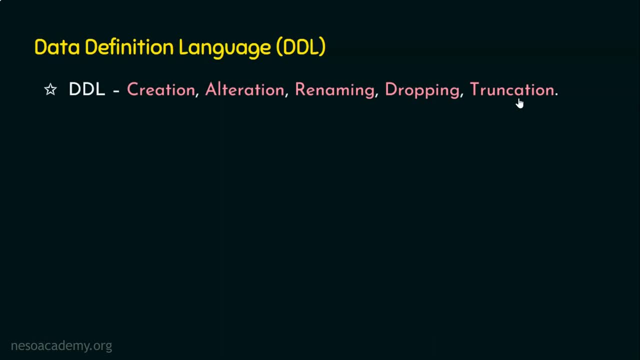 the table, but the schema remains. the structure remains. Drop deletes everything, whereas truncate deletes only all the data present in the table, but the table structure exists. The schema will still persist, but it will remove all the data present in the table. So again, this is also DDL data. 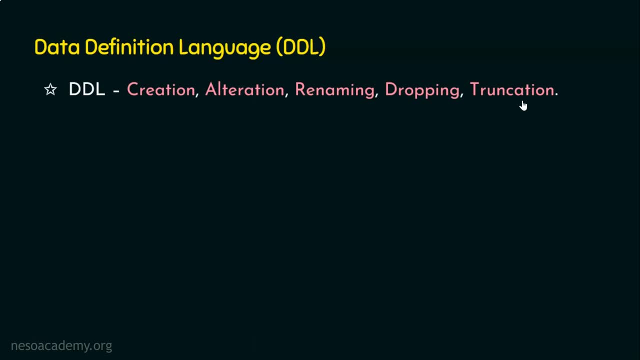 definition language. I hope now you understood why do we need two separate languages. The first language, DDL, deals with the schema, And the second language, DML, is going to deal with the data part. Now, what are all the additional information that we are going to see in DDL? 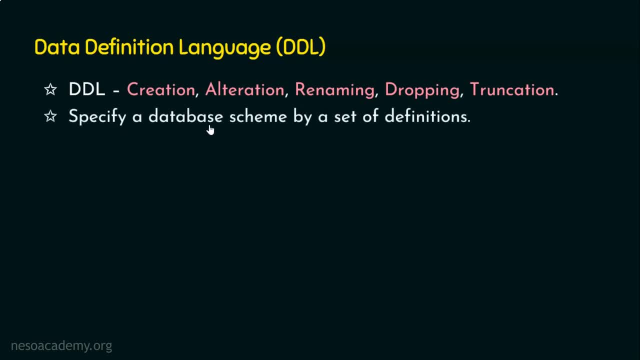 Actually, this DDL is used to specify a database schema by a set of definitions. Say, if we want to create a table or alter or rename or drop or truncate, everything is a specification of a database schema by a set of definitions, And that is why. 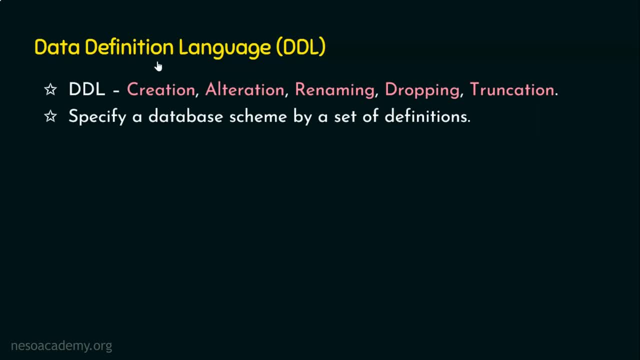 we call this language as a definition language, which is a data definition language- DDL- And while creating the database schema, we may include some consistency constraints. What do we mean by consistency constraints? Let's take it is a bank database and there is a column in the account table. 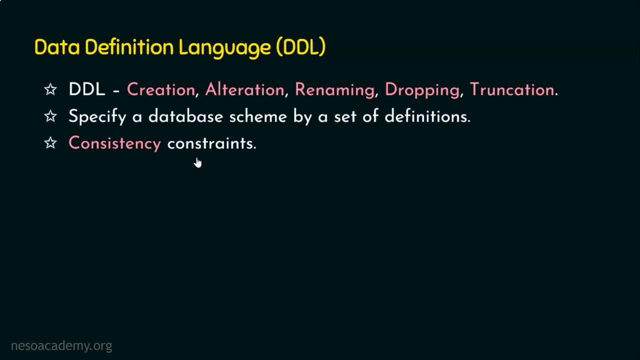 where the balance column should not be lesser than or equal to zero. In that case, we are enforcing a constraint to the schema that, whenever we try to insert a new data into the table with the column, account balance is equal to zero or lesser than zero. 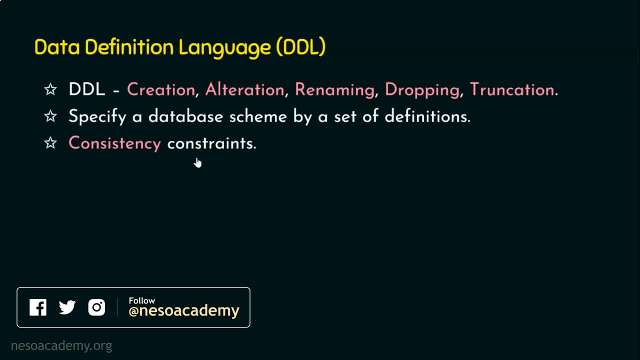 The database should not accept that, because we have enforced a condition or a constraint to the table: that balance column should not be lesser than or equal to zero, And this is one of the constraints. and likewise we can enforce a lot of consistency constraints so that we can make the database a powerful and a 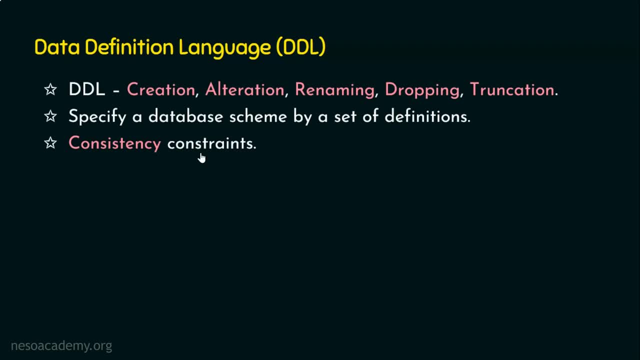 consistent one. So this consistency constraints can be enforced on the database in two ways. One is with the domain constraints and the other one is the referential integrity. Firstly, let's focus on the domain constraints. Let's take a table. in a table will be obviously having some columns. 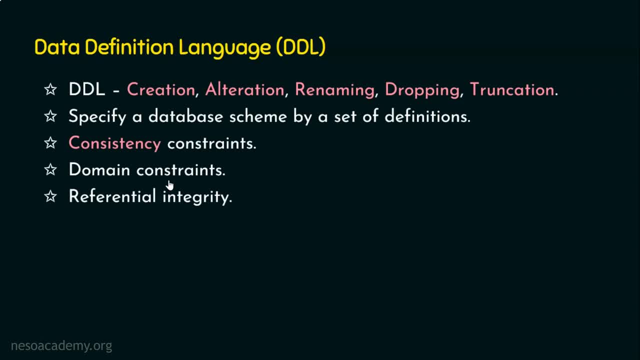 Each column is specified by a data type. This itself is a constraint to some extent. Let's take an example: Employee table. The first column is ID, I mean employee ID, and employee ID is all of numbers. In that case, we are specifying the data. 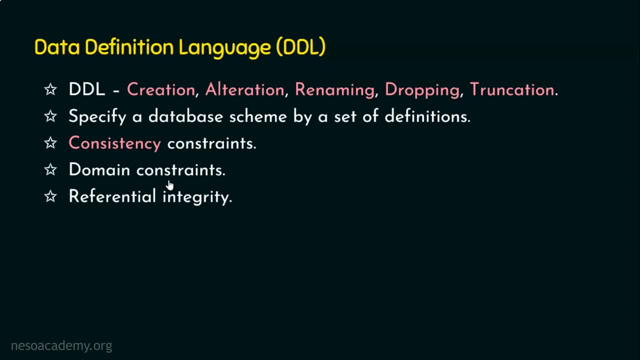 type to the employee ID column as numbers. After specifying the employee ID column as a number type, I mean the number data type Thereafter, whenever we try to insert some records into the table. if the employee ID columns is only of numbers only, then that insertion or updation will be accepted. 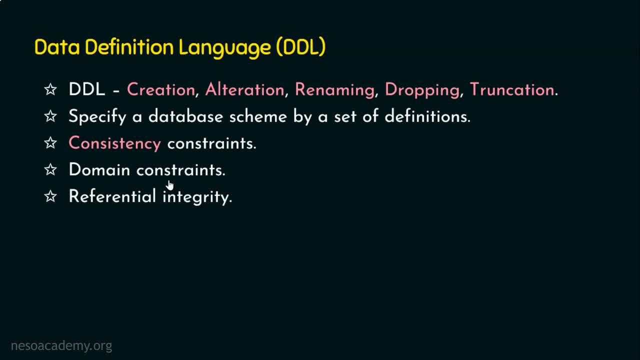 Otherwise, if we try to insert some date data type or character data type into the employee ID column which is set as number type, it will not accept And this is one of the constraints that comes under domain constraints. Specifying a data type itself is a domain constraint. 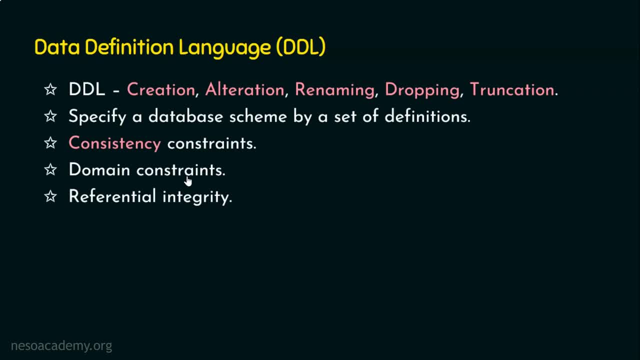 And also we are enforcing some conditions to the columns, like account balance should not be lesser than or equal to zero. This is also coming under domain constraints only, And talking about the second one, the referential integrity constraint, Suppose we are inserting a value into the table and that value should exist in other. 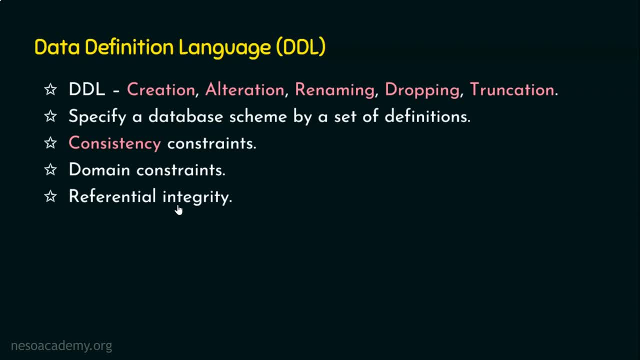 table. We are referring the value which is inserted in one table and we are specifying a condition: that that value, whatever we are going to insert into the table, that value, should exist in another table. Here we are referring another table. Only when this condition is satisfied, this operation will be accepted. 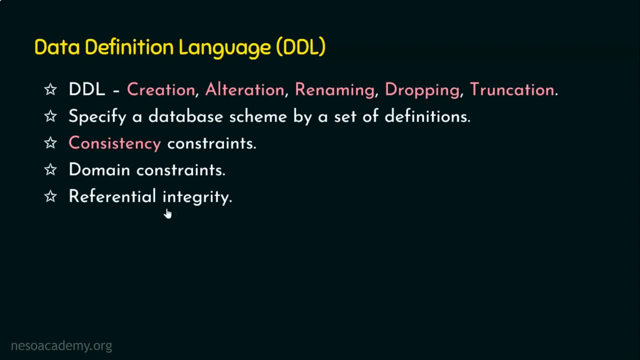 So this kind of constraint is called as referential integrity. Don't worry about this. now, In the coming chapter, SQL, we are going to focus exclusively on all the features of the language, where we are going to exclusively focus on the domain constraints and the referential. 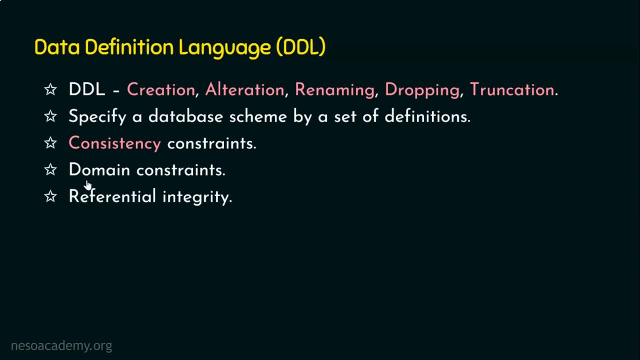 integrity with examples For now just understand: If it is a domain constraint, This is restricted to the table. It can also be a referential integrity, where a table is going to refer another table. Basically, these two types of constraints are special type of constraints that can be: 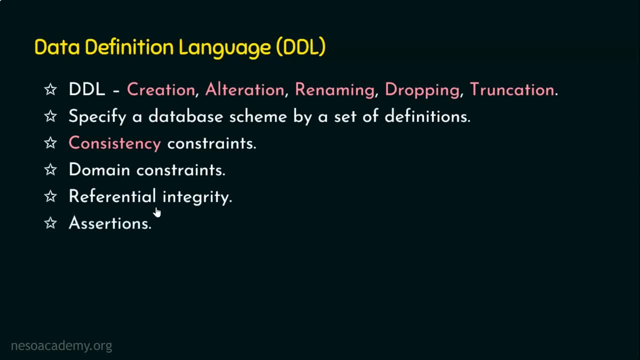 defined, along with the table itself. But there are situations where we cannot express our conditions using domain constraints or referential integrity. Those things can be expressed using assertions. So assertion in DBMS is any condition that the database must always satisfy. In coming to the next point, which is authorization, this authorization simply means that who can 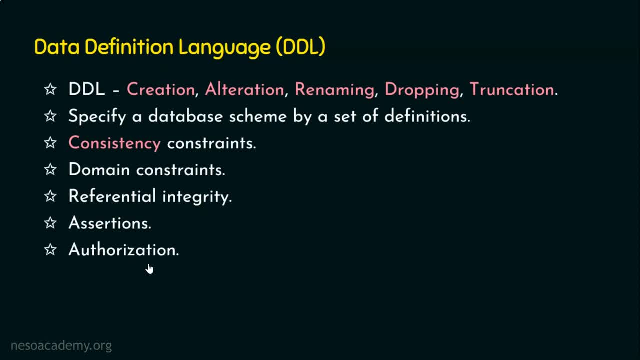 access what data item. Generally, authorization deals with the privileges held by the user who accesses the databases. Authorization can be read authorization, insert authorization, update authorization or delete authorization. Say, if a user is having read authorization, he can read the data present in the table. 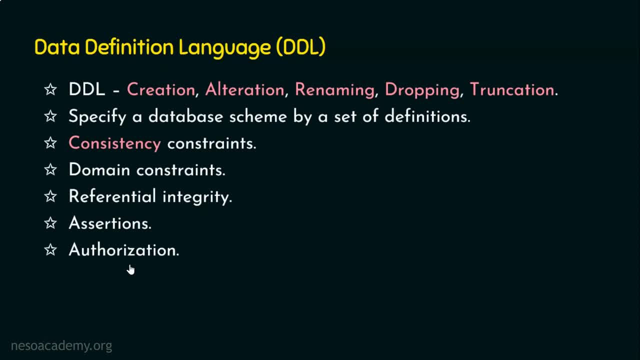 but not write. If a user has insert authorization, he will be able to insert authorization and do read, but not write records into the database. If he has update authorization, he can update the database. Suppose, if a user wants to delete some data present in the database, then he should have. 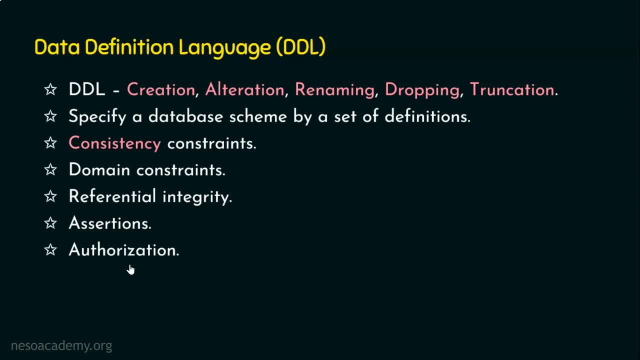 delete authorization. So we may assign all or none or even any combination of these types of authorizations, like read, insert, update or delete authorizations. And coming to the last point here, the data dictionary and the metadata. What do we mean by data dictionary Generally, whatever the 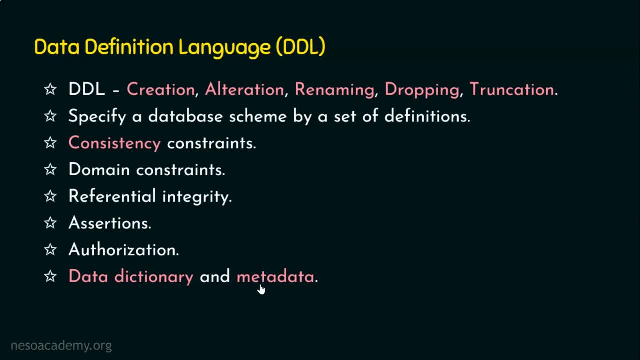 DDL commands. we execute all these DDL commands is going to generate an output, And the output of all the DDL command is placed in a special table called data dictionary. Remember this data dictionary is a special type of table And what this data dictionary table is going to contain. 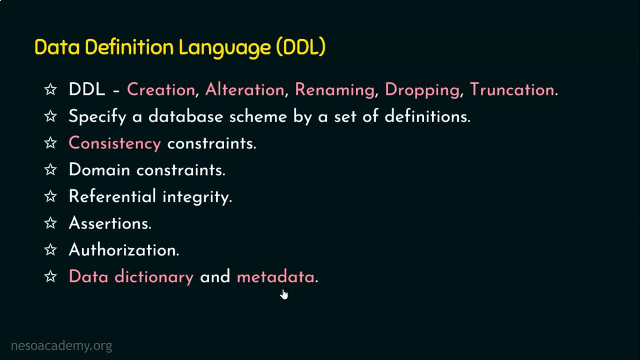 It's going to contain metadata. It means data about data. So data dictionary is a special type of table that can be accessed and updated only by the database system and not by the database itself. So data dictionary is a special type of table that can be accessed and updated. 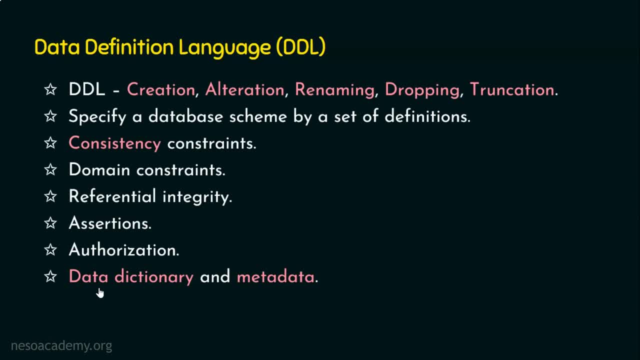 by the regular users of the database, And that is why I referred this table- data dictionary- as a special type of table, because it can be accessed and updated only by the database system. Also, it contains metadata, which is data about data And whenever any operation is carried out on the 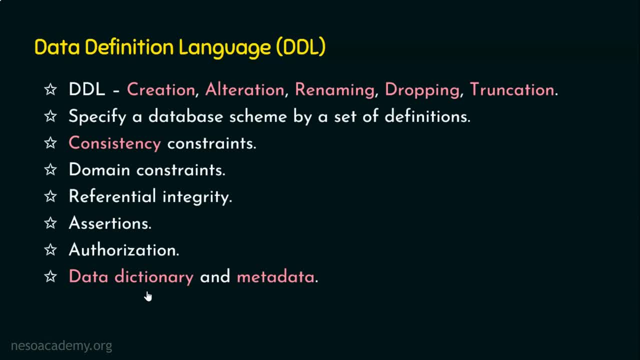 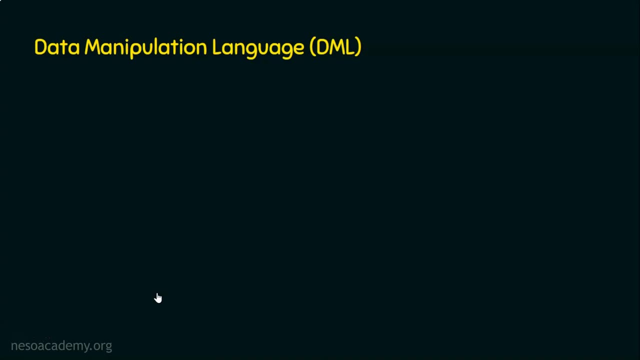 database. the database system always consults this table, the data dictionary, before reading or updating the data in the database. We are done with the first language, the DDL. Let's now focus on the second one, the DML. We are aware that DDL, the data definition language, deals with the schema. 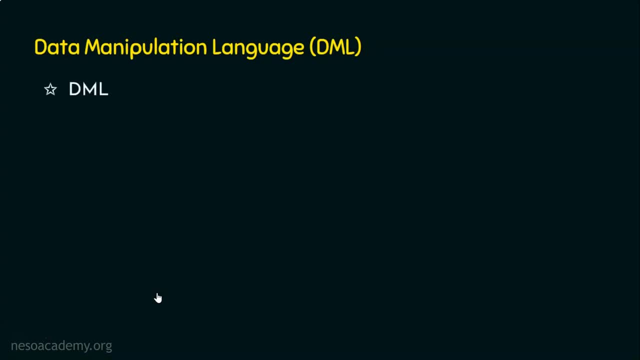 And this language, DML, data manipulation language, which deals with the data present in the table, Say, if we want to see what role the data present in the table, so retrieval is the option, So retrieval of data, or inserting data into the database or deleting the data from the database. 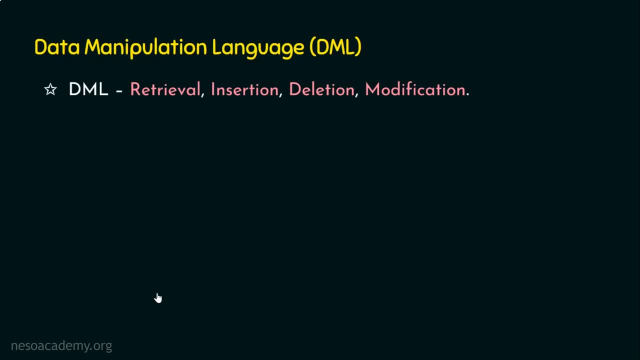 or even modifying the data from the database. all these operations are coming under DML, the data manipulation language. Remember, here only data part is dealt and DML does not deal with the definition or the schema. Let's assume there is an employee table and we want to see all the data present in the employee table. 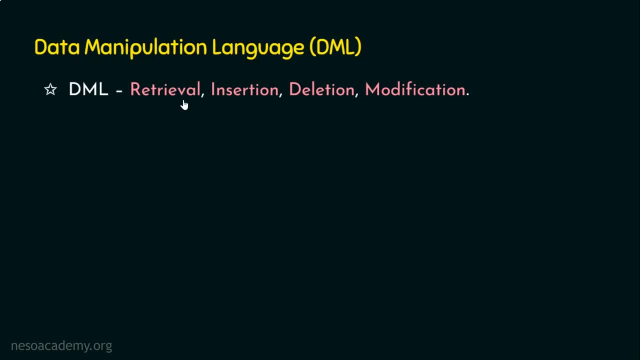 So we can retrieve the data using DML statements And if we want to insert a row into the table, that is also DML only. We want to delete or modify the existing data, this is also DML only. So, in simple terms, DDL deals with the schema and DML deals with the data And basically we 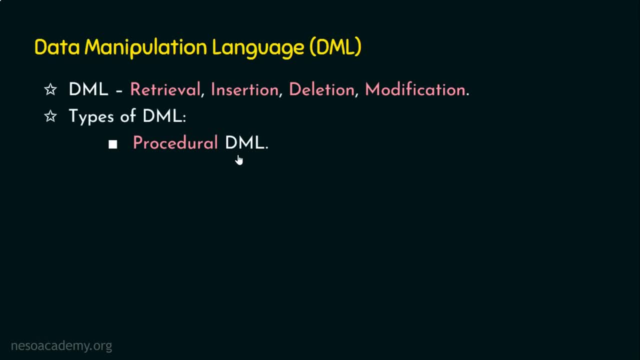 have two types of DML. Number one, procedural DML, and number two, declarative or non-procedural DML. Procedural DML means we need to specify what data is required and how to retrieve those data, Whereas in non-procedural, we are simply going to specify what data is required. 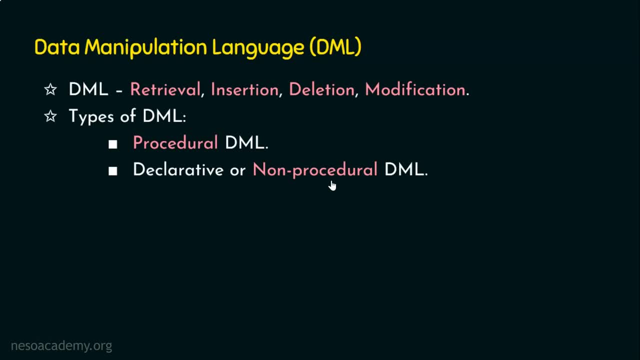 and how we are going to retrieve the data. We need not specify that. Anyway, in the coming lectures we are going to focus on procedural DML and non-procedural DML. elaborately, If we write a statement requesting the retrieval of information. 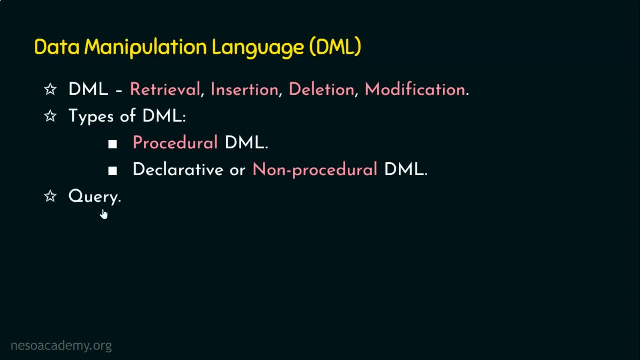 we call that statement as a query. So if we write a DML statement that is requesting the retrieval of the information from the database, then that statement is referred as a query And generally the query language and DML are used synonymously. So before we sign out: